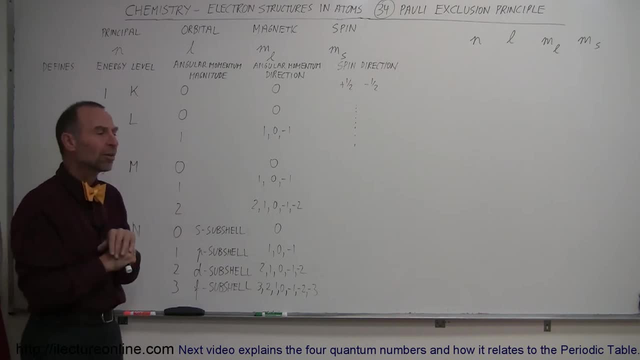 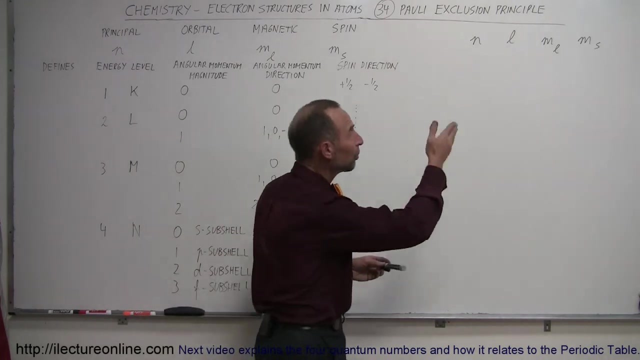 so another way of looking at the Pauli Exclusion Principle is that you could only have a maximum of two electrons in each orbital and only if the two electrons had opposite spin- another way kind of looking at the Pauli Exclusion Principle. So as an example, let's say we'll start putting down electron configurations. 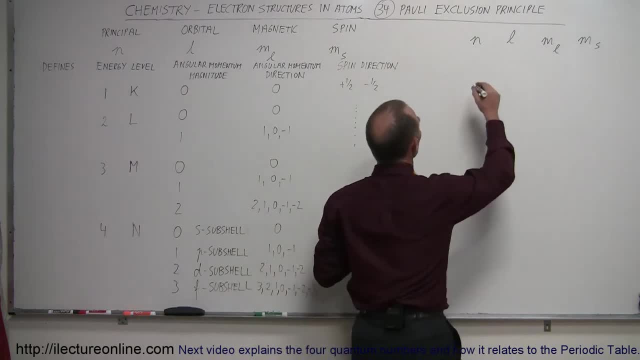 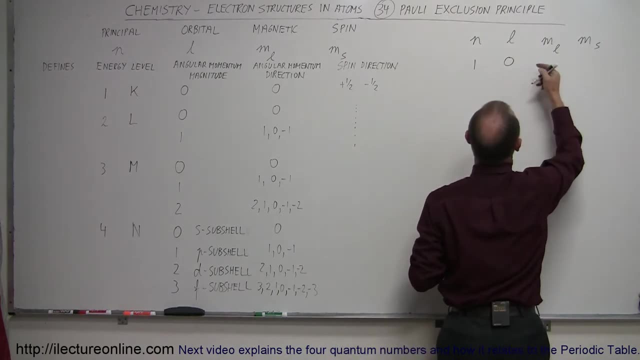 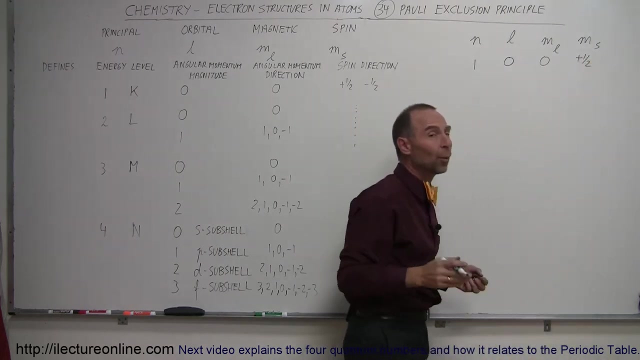 based upon this principle. So let's say we talk about electron being the first energy level which necessitates it to have zero angular momentum quantum number and zero magnetic quantum number and either a plus or minus one-half spin number. So let's say one electron has those four quantum numbers. 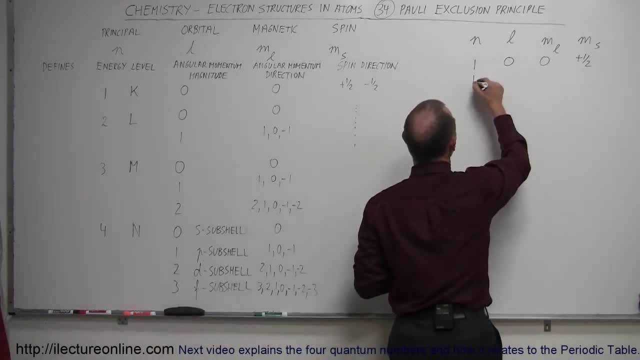 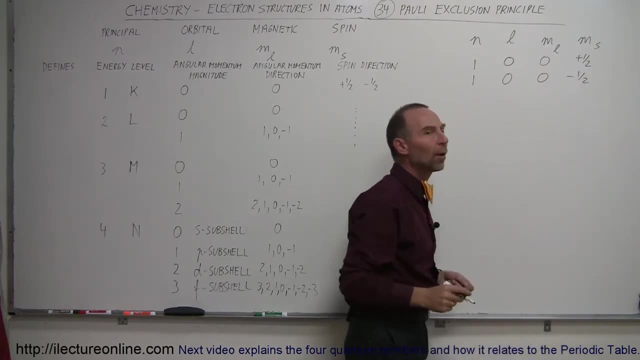 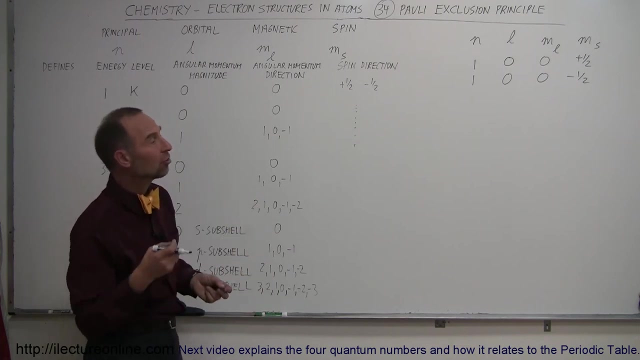 then the other electron in the same energy level, with the same angular momentum, in the same angular momentum direction, would have to have an opposite spin direction. Now that represents the first s-orbital in the first energy level. That one is now filled with two electrons, and so any additional electrons added to the atom. 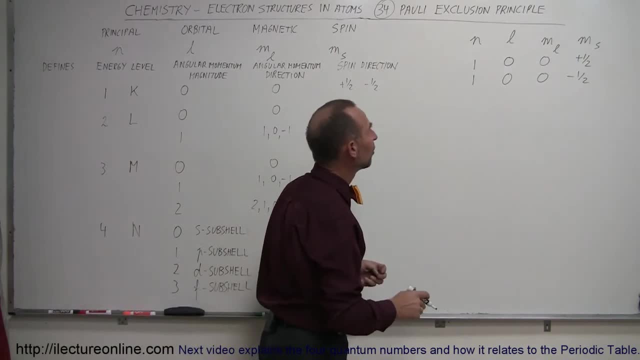 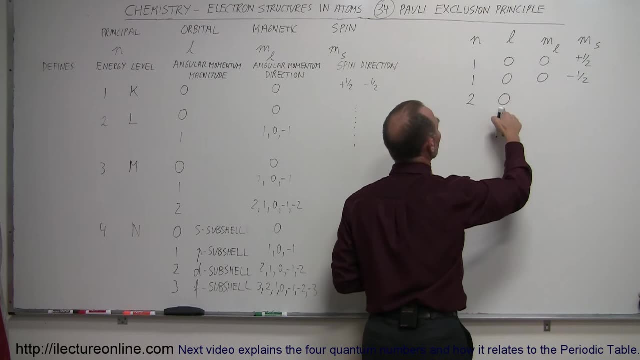 now has to reside in a different location because it cannot have the same quantum numbers. So then the next electron would be in the second level, perhaps in the zero orbital level, which would be the s-orbital with a zero spin direction. 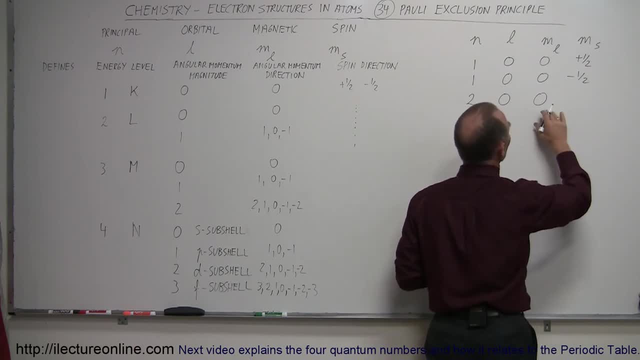 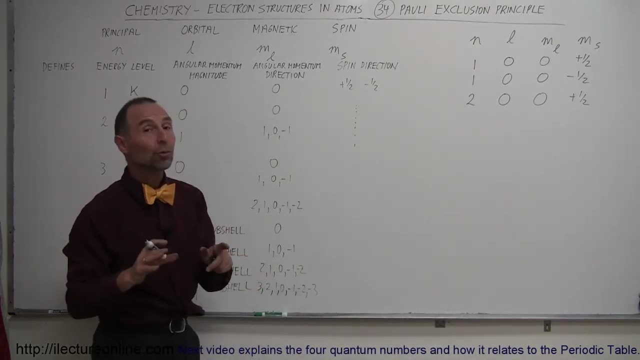 or I should not say spin direction, but angular momentum direction and maybe a plus one-half spin direction. So that is the s-orbital. in the second energy level There's room for a second electron, but that electron has to have a different set of quantum numbers. 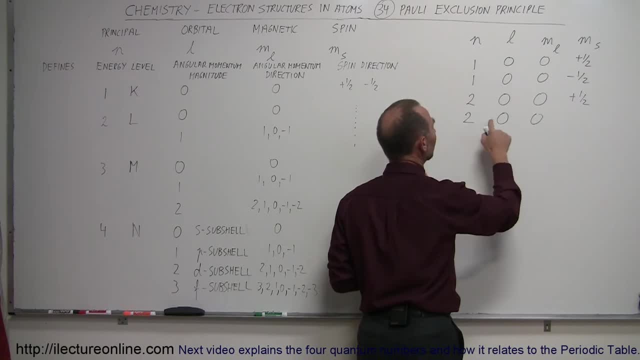 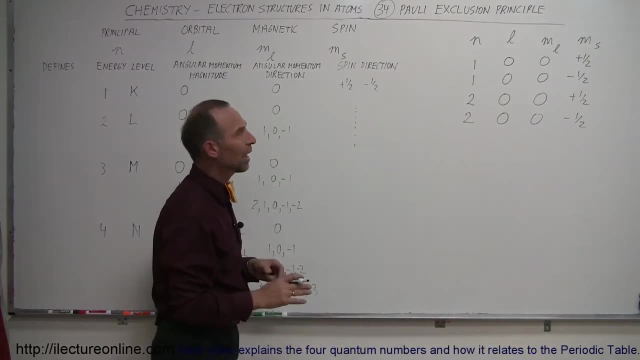 It could have the first three quantum numbers, the same second energy level, That would be in the s-sub-shell, the s-orbital, and that would be in the minus one-half spin direction. So now we have the second orbital filled up. 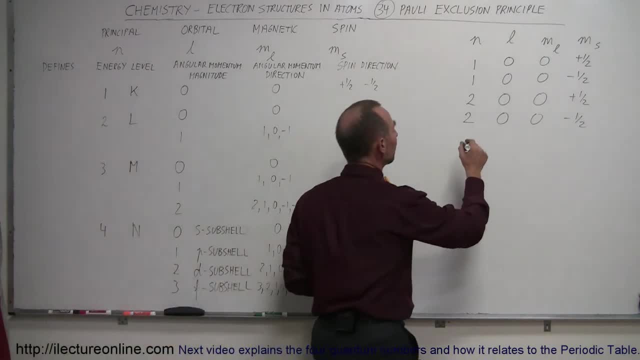 The next electron would have to have different quantum numbers. It could still be in the second energy level, but now you would have to be in the p-sub-shell. That means it has a different angular momentum. It could have a possibility of three directions: spin directions. 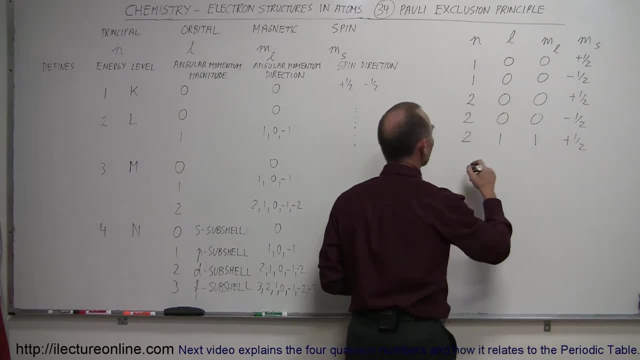 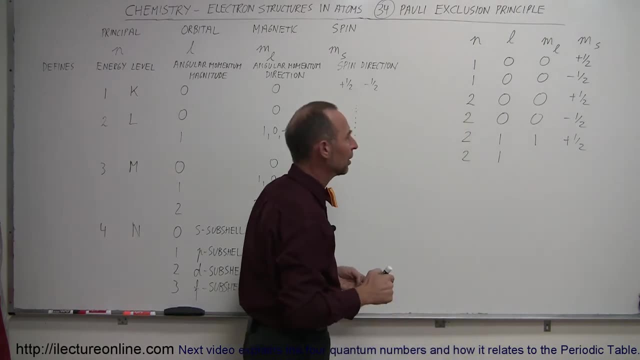 So let's say, call this one and call this plus one-half. The next one would have an energy of two. It may still be in the same. well, if it's in the p-orbitals it would have the same angular momentum. Perhaps same direction, but then it would have to have a different spin direction. So it would have to have, if it has the same angular momentum and the same angular momentum direction, it would have to have a different spin direction in order to exist in the same orbital. 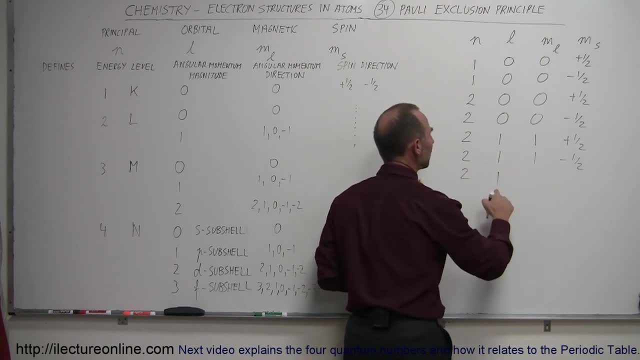 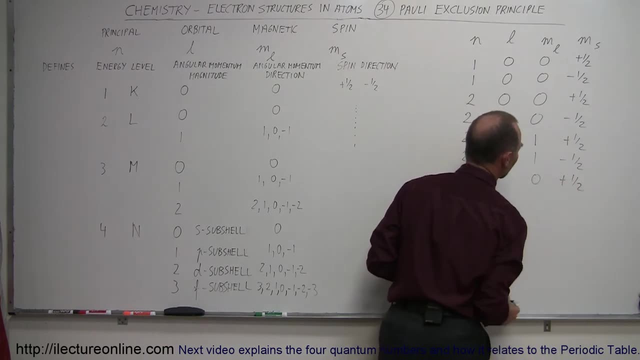 Going on. we have again same energy level, same p-orbital, shell, sub-shell, and then we have a different p-orbital and a spin direction of plus one-half. And if we have a second electron that exists in the same orbital, 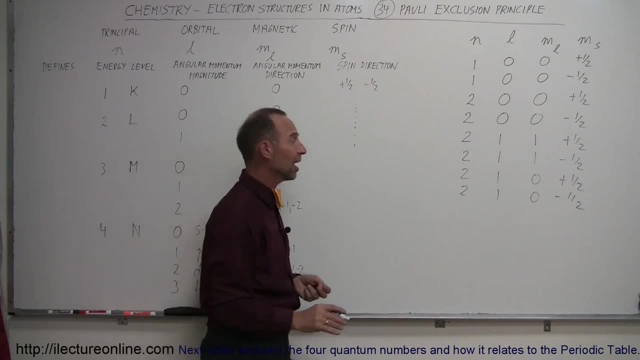 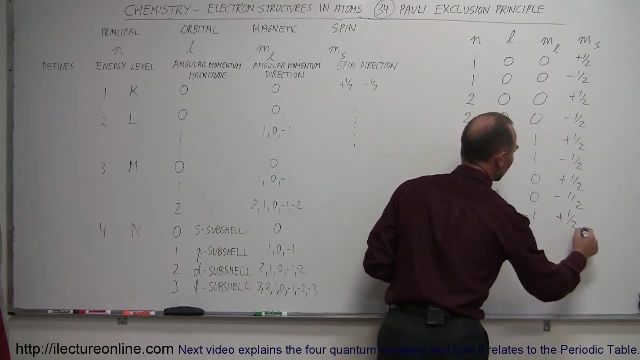 it would have a spin direction of a negative one-half, Still in the same energy level. there's still a third p-orbital, Different spin direction, Or I should say not spin direction but a different angular momentum direction, And then, of course, a spin direction like that: 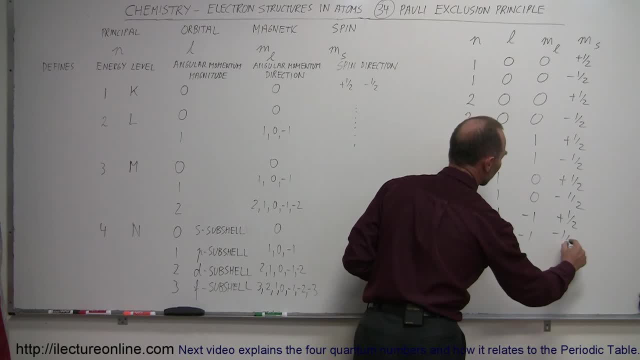 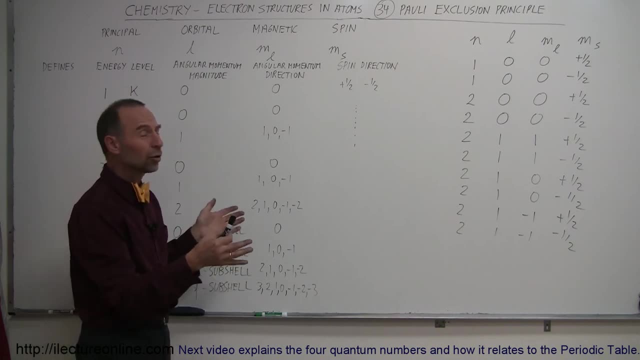 And if a second electron appears in the same orbital, it would have to have a different spin direction, and so forth. So Pauli understood that electrons are situated around the nuclei of an atom in such a way that in no circumstance would an electron have the same properties. 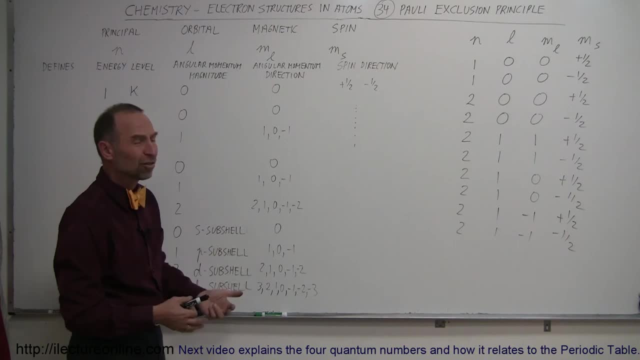 of energy level, angular momentum, angular momentum direction and spin direction all at the same time. So therefore, electrons are filling out those orbitals around the nucleus in such a way that they're neatly stacked with their own unique set of quantum numbers defining the properties of the electrons in those locations. 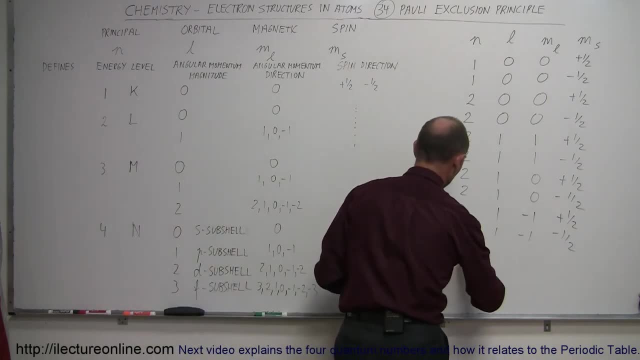 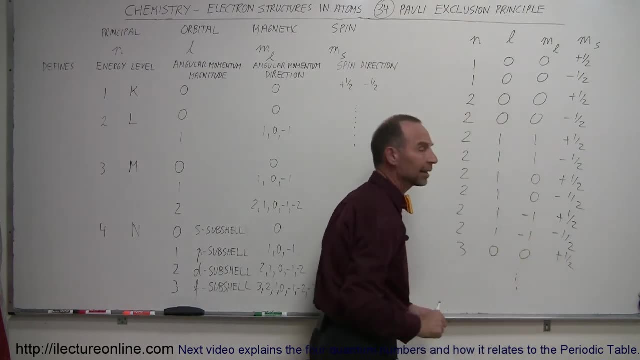 Of course the next one would be three Third energy level, s-orbital zero for m-sub-L, and then plus one-half, And of course we continue on like that Again any time you add another electron, different set of quantum numbers.